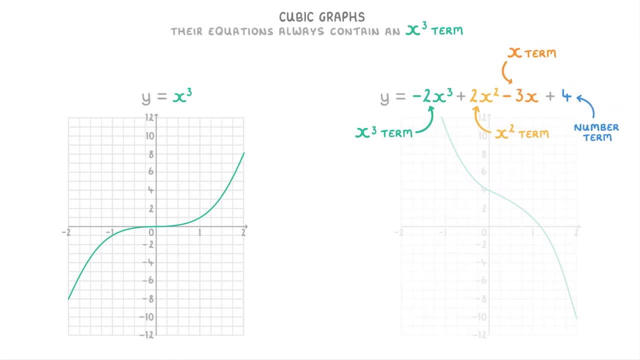 a number or integer term. In general, we can say that their equations will look something like this, where a can be any number other than 0, and b, c and d can be any number including 0. So basically all that means is that cubic equations have to have an x cubed term, but 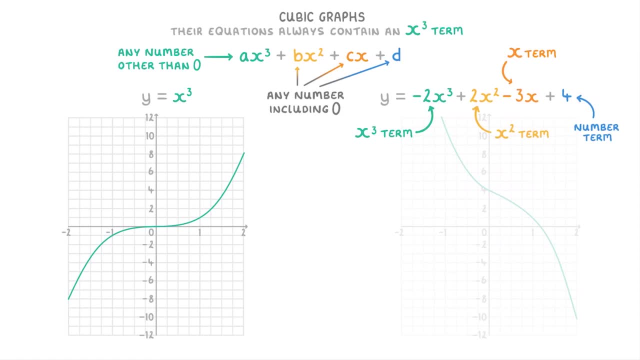 may or may not have an x squared x or number term. So something like x squared plus 2x plus 1 doesn't count as cubic because it doesn't have an x cubed term. And x to the power of 4 minus 2x cubed plus 1 also doesn't count as cubic because it. 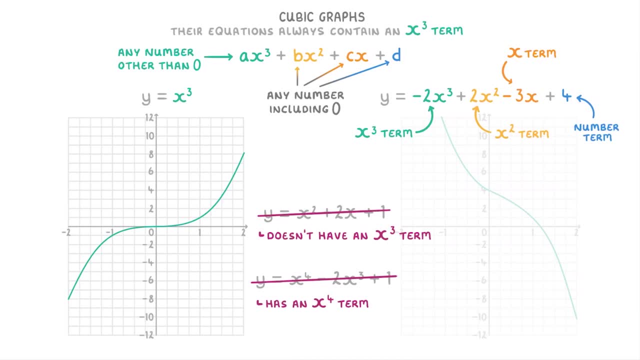 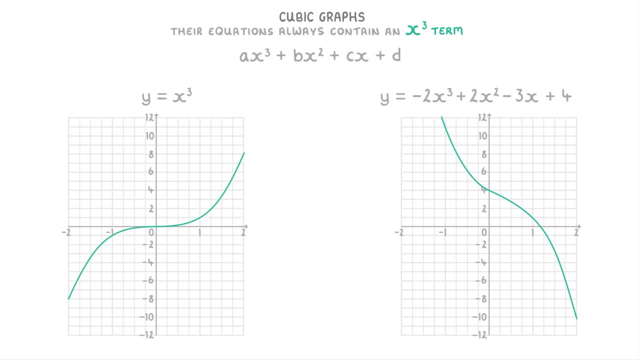 has an x to the power of 4, term which isn't allowed. Now you don't need to be able to figure out exactly what a cubic graph will look like just by looking at the equations, But You can also know whether it will go from the bottom left to the top right or from. 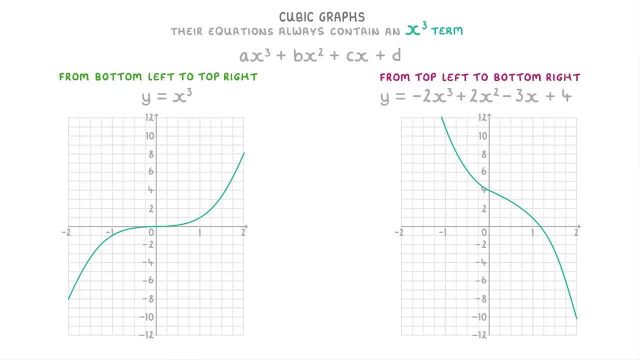 the top left to the bottom right, And you can tell this from whether the x cubed term is positive, like it is for y equals x cubed, or negative. One way to remember this is that if you draw them from left to right, positive cubic graphs. 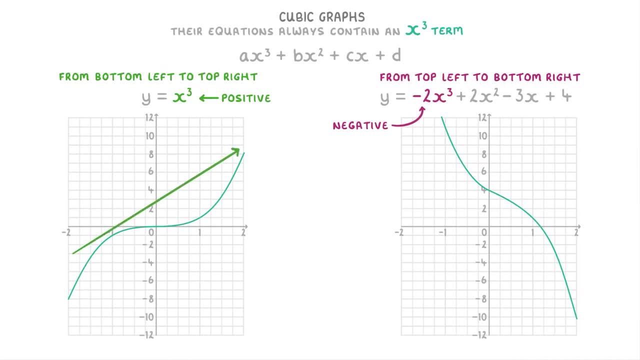 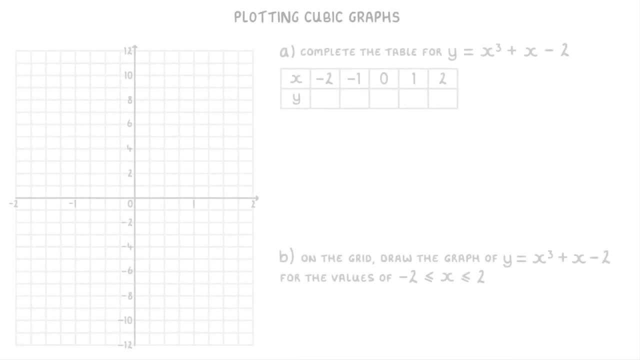 go up because they're positive and negative. cubic graphs go down because they're negative. Then get this thing done. We'll plot these cubic graphs And we'll use this question as an example, which is about the equation y equals x cubed. 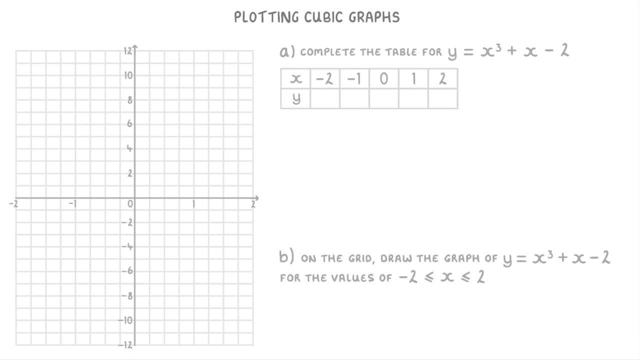 plus x minus 2.. Now, just like when you're plotting linear or quadratic graphs, the first thing you need to do is complete a table of x and y values so that you know some of the points that the graph will pass through. And then, once you've done that, 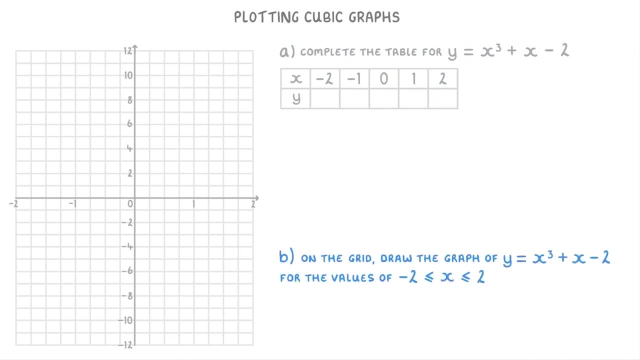 Then You're done. you can plot all of those points on a graph and join them up to get our curve. So to fill in the table, we need to figure out what y will be when x is each of these values. So to find y when x equals minus 2, we just plug minus 2 into the equation that we were given.